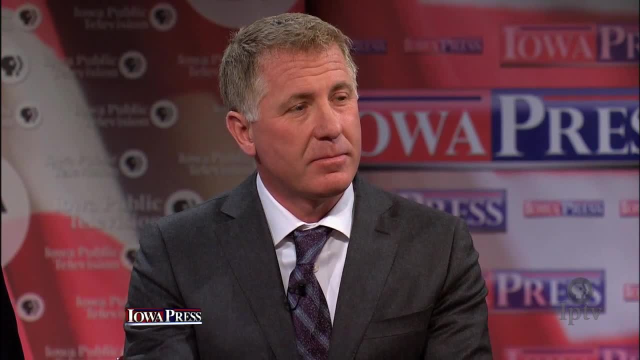 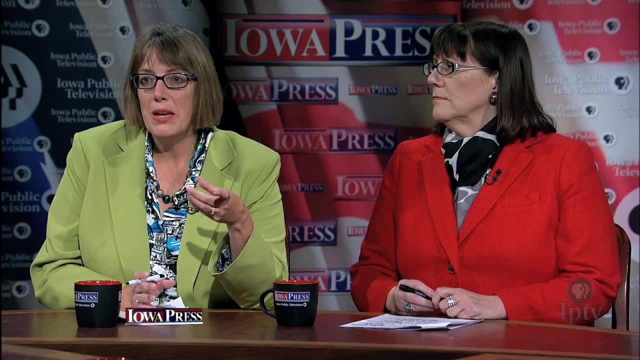 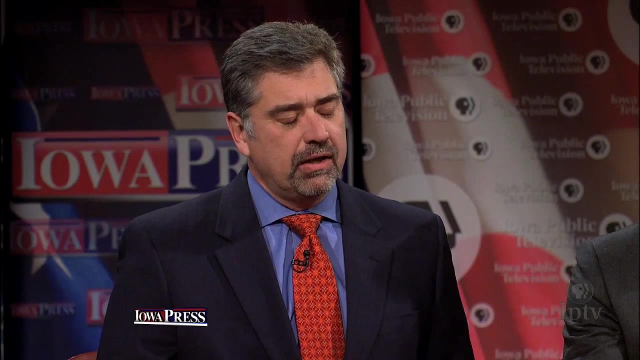 Republicans ate into the democrats historic early voting advantage this time. How are democrats going to innovate or renew their advantage in 2016?? Well, it's an interesting question and I've looked at this a little bit. We won't know, really, until December, when we get the voter file back to see who voted and who didn't. 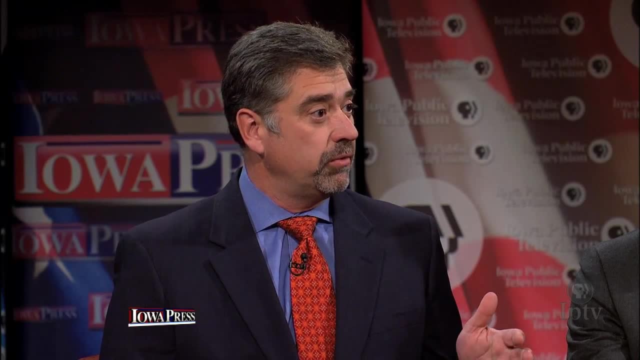 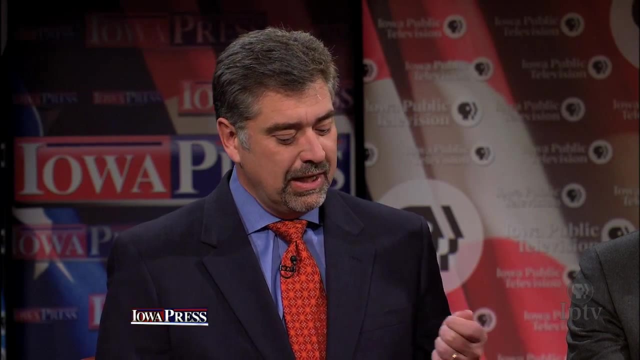 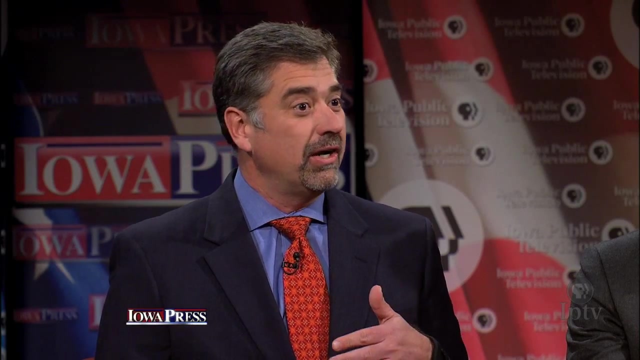 But early vote was larger for both parties this time. In fact, there were 121,000 more early vote requests in 2014 than in 2010.. And there were 114,000 more early votes this time than in 2010,. yet the turnout wasn't larger. We had 100,000 people that shifted to early vote. 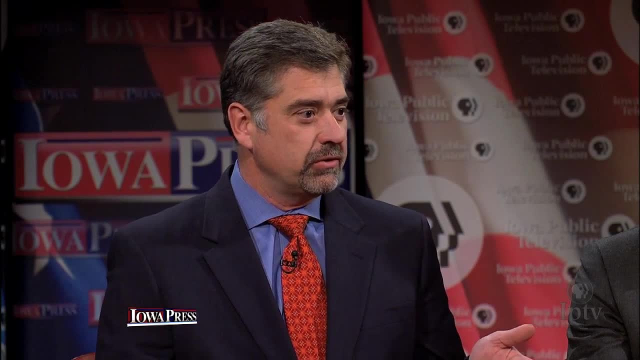 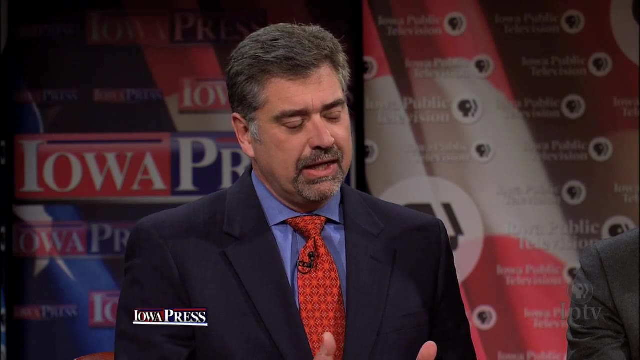 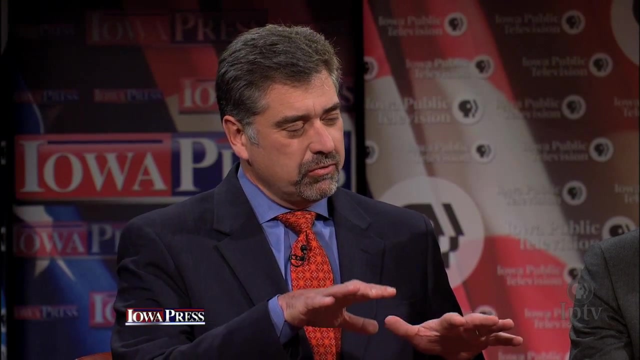 And, if you look at it, the democrats, I think, had 34,000 more requests. the republicans had 45,000. So they increased by about a quarter. We had about 11,000.. I think what happened, though, if you have 100,000 or so more early voters and the parties were roughly at parity. we had a lot of democrats that sat home, who are good voters. 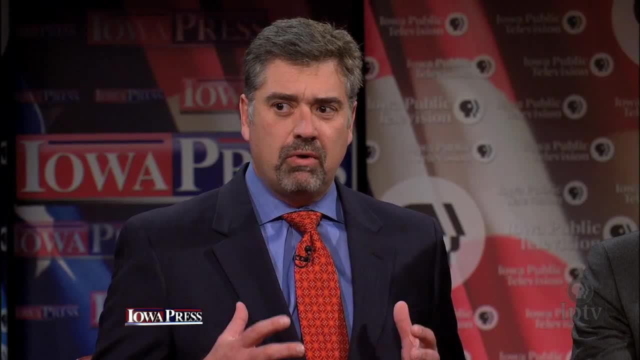 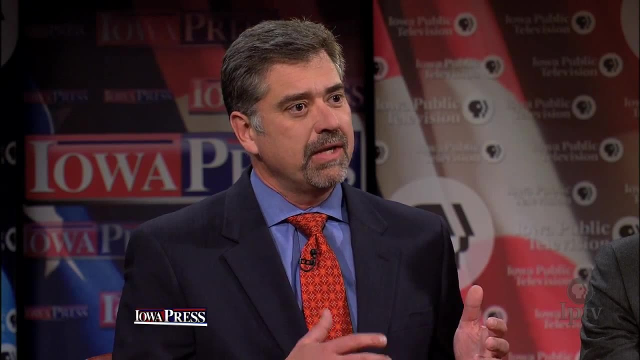 And so that's what we really have to look at and say: why did these democrats who voted in 2010 maybe sat home this time? And I think again, it's a combination of message. You have to give people a reason to show up and vote. 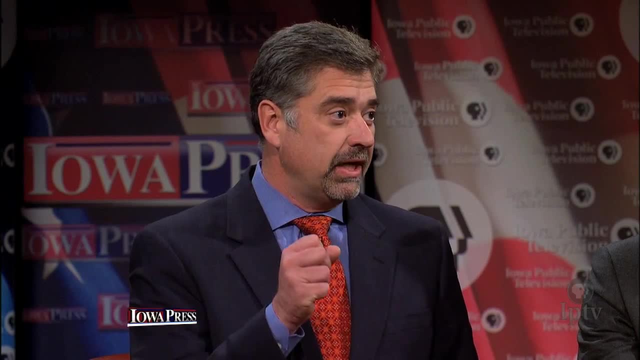 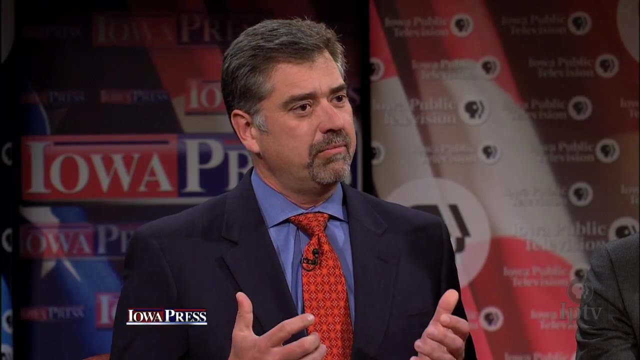 We had a terrific election. We had a terrific field operation. We had people knocking on doors, I think we had volunteer shifts filled all around the state. We had a terrific mechanical operation, but we needed to have a message to marry with the mechanics. 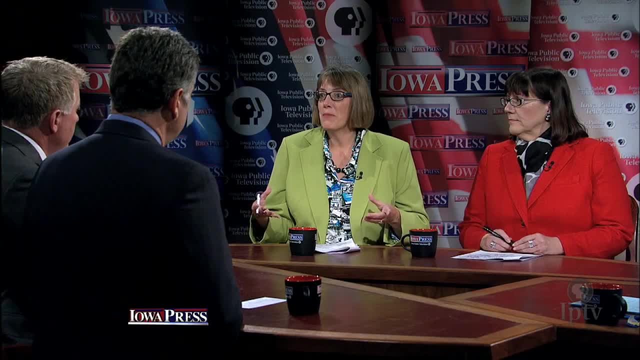 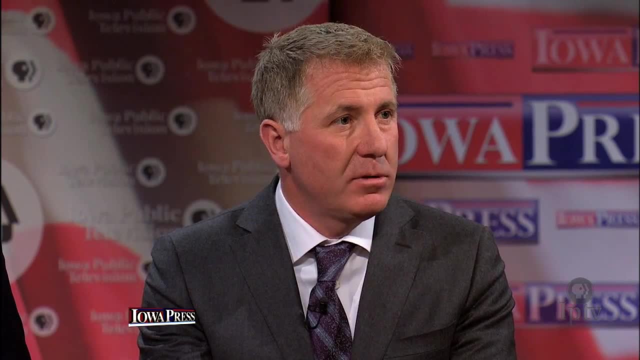 And David, is this a once and for all that republicans have overcome their resistance to early voting, or is this something you're going to have to battle every election? We're going to have to battle every election. What we did this time was a lot smarter, a lot more targeted, more focused. 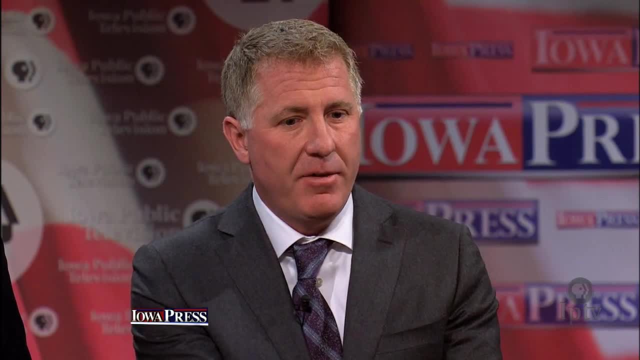 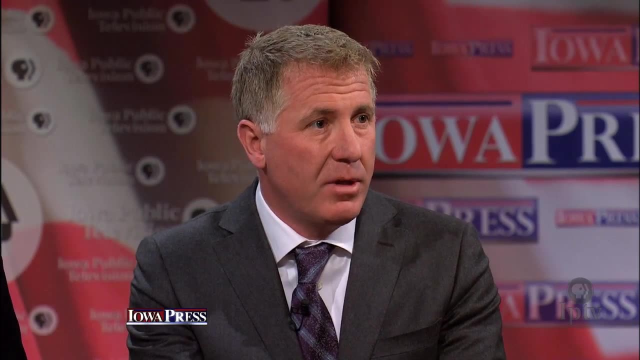 We did very much overperform where we've been in the past. What democrats did is they left about 20-some thousand ballots on the table that didn't get turned in. Republicans didn't do that. We performed our ballots.